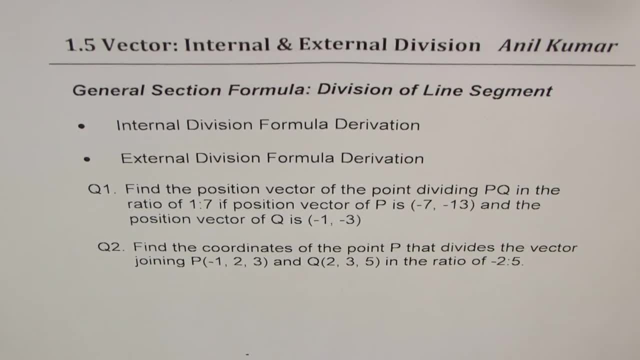 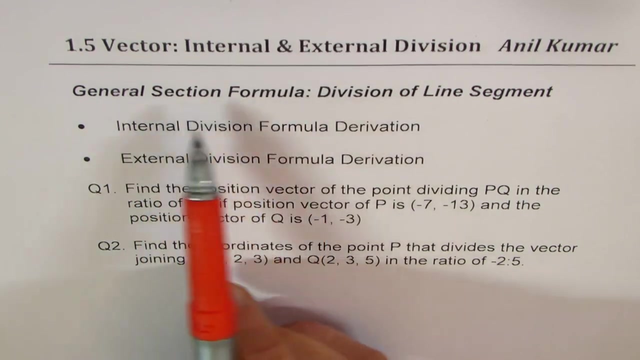 I'm Anil Kumar. Welcome to my series on vectors. Now, in this particular video, we'll apply our learnings of scalar, multiples, linear combination and understand how to find general formula for internal and external division of vectors, And we'll take up two examples, as mentioned here, to understand our learnings. So we'll begin by deriving a formula, which is also referred to as section formula: division of line segment. 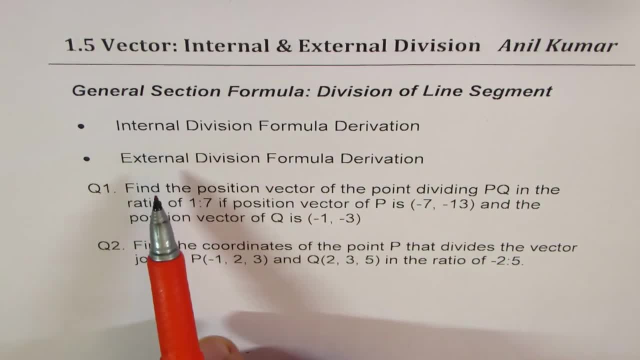 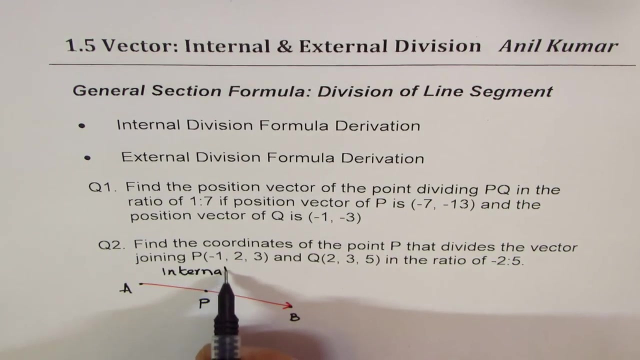 Now a line segment could be divided internally or externally. Let's understand this first. Let's say: if I have a vector here, Now let's call this vector as AB And let's take a point somewhere in between. In that case P divides the vector AB internally, So this becomes internal division. Is that clear? 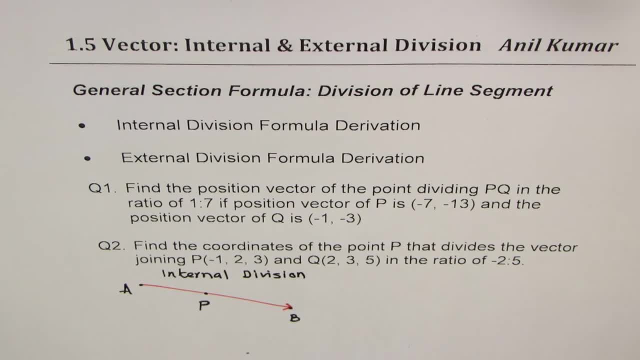 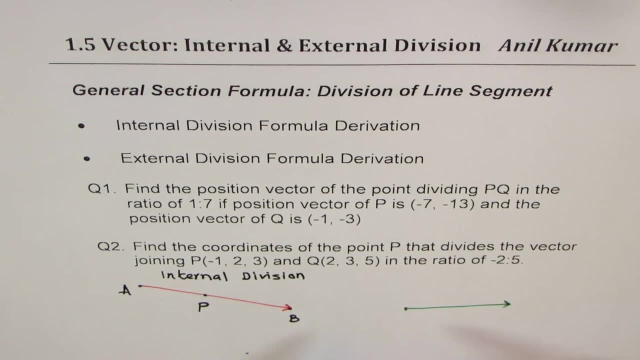 Now, on the other hand, we could have something like this: Let's say that the line is A to B, But the point is point P is somewhere here External to the line. That means we have A to B right Now. point P still divides the vector AB into two parts, But this time P is outside AB, right? 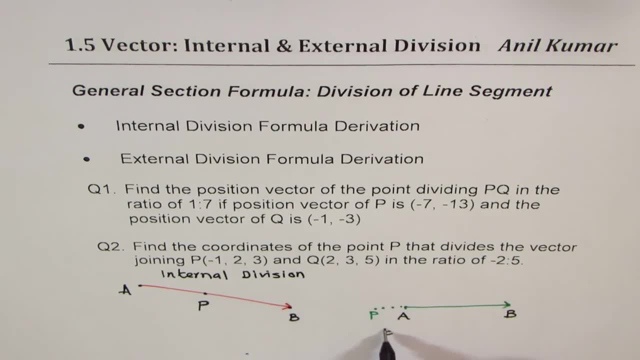 So we'll consider both the cases Now here, when we say A to P and then P to B, we write: the ratio AP is to PB, right, Both are positive, Do you see that? But in this case A to P is negative, And then from P to B. So that is the kind of figure we have. 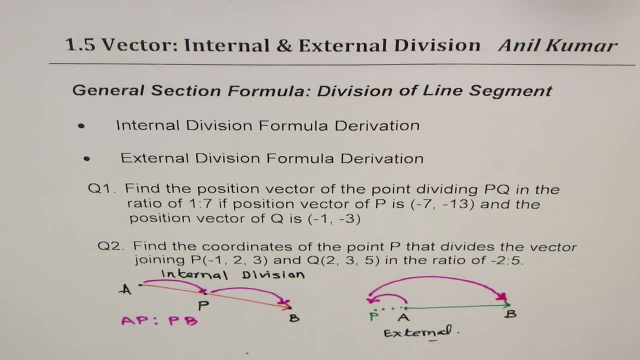 So you could say that in one case we're considering both positive. Let us say we have a ratio of 2 is to 3.. In this case we could say is a ratio of, let's say, minus 2.. Bringing it to this side and let's say 7.. Going there, 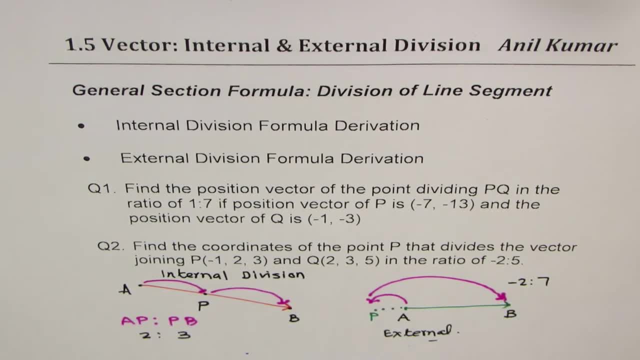 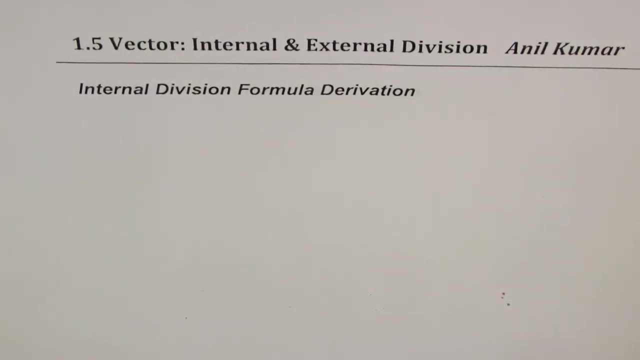 So that becomes external. So I hope that point is well taken care of. Now, when you understand what we're trying to do, Let's begin by deriving a general formula of solving such questions. So we'll take up internal division first. So let's again take a line AB. so let me just sketch a line here. 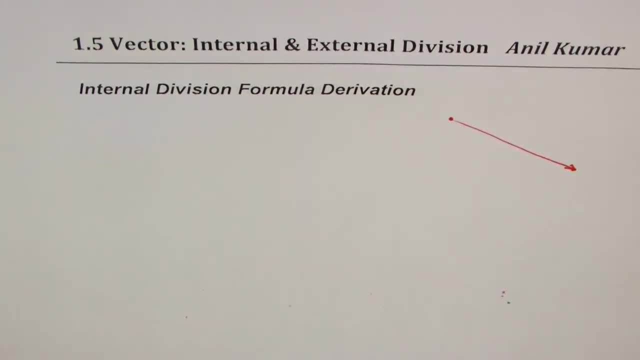 When I say line, I mean vector actually, So vector which is directed from A to B. Here we have a point P somewhere in between, which divides the vector in two parts, so A to P and from P to B. Let us say these parts are M and N, So that becomes general division. 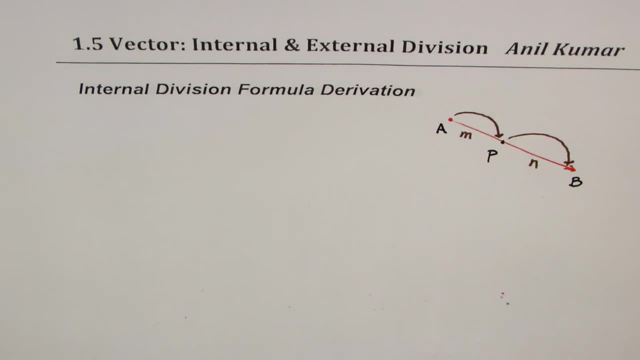 of line. Since P is in between A and B, we'll call it internal division. Perfect, Now let us draw a coordinate plane also. It becomes simpler to visualize in this fashion And to make things simple, I'm considering the vector in our quadrant one. 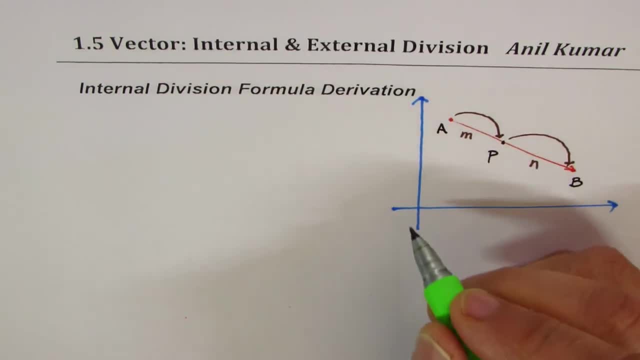 Now, what is a position vector? Position vector is vector with respect to origin O. So if I join OA, OA becomes a position vector, OP is a position vector, OB is a position vector, Is it okay? So OA is a position vector, OP is a position vector and OB is a position vector. 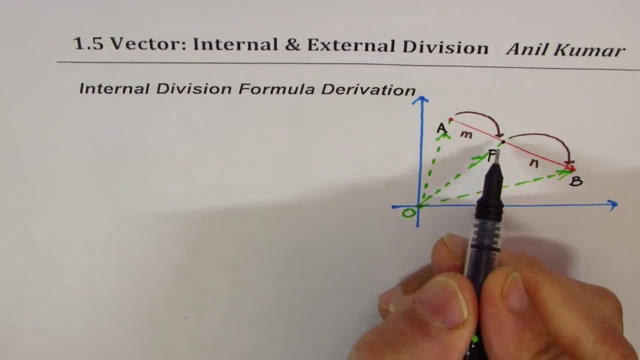 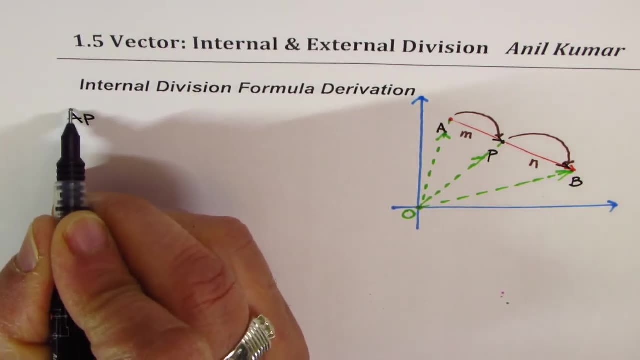 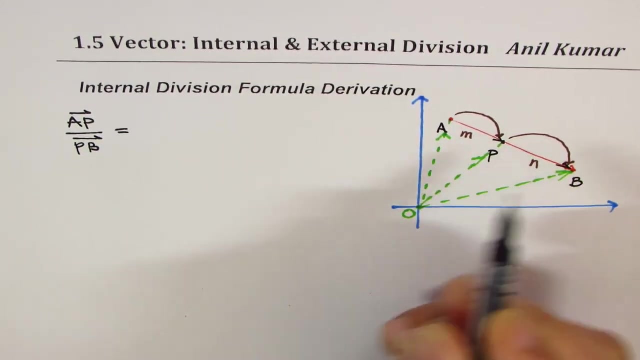 Now, since we have AB, all are going in the same direction. right, they are all going in the same direction. We can say that the ratio AP is to P to B is, as given to us, M over N. right, The magnitudes are different, their direction is same. 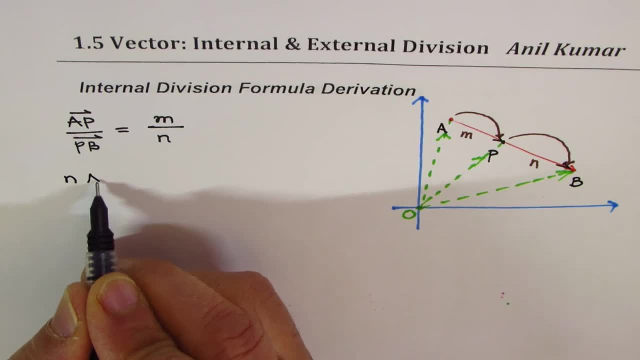 So we can now cross multiply and write this as N times AP is equals to M times PB. Just cross multiply, Okay, Okay, Just cross multiply. We're using the properties of scalars. They could be, you know, all this can be done with scalars, all these mathematical operations. 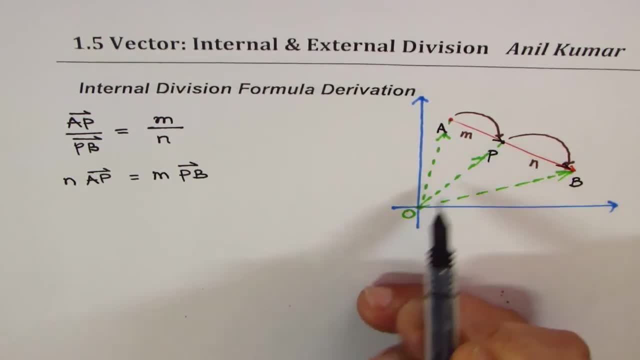 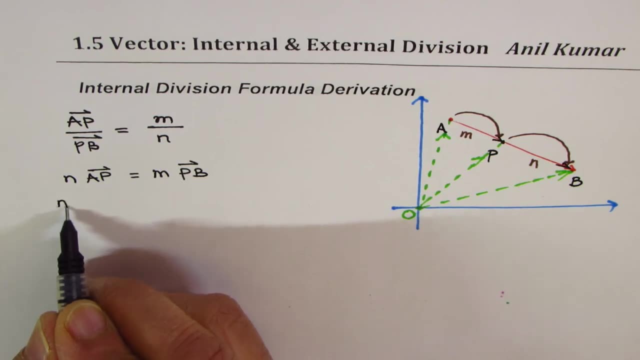 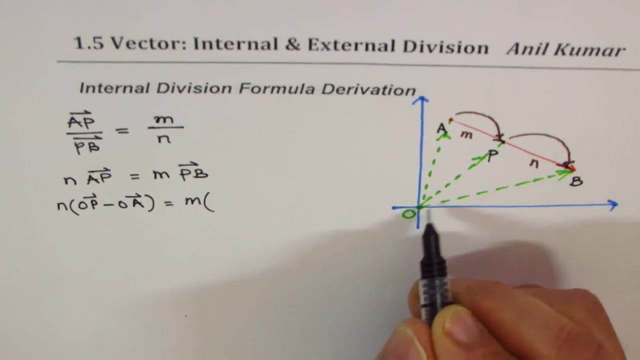 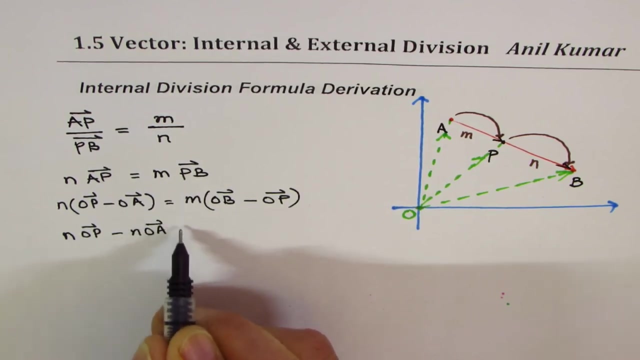 right Now. what is AP? So if you look at the position vector, AP is OP minus OA. So I replace AP by OP minus OA. Similarly, PB is OP. Okay, Okay, So PB is OB minus OP. Now we can open the brackets. N times OP minus N times OA equals to M times OB minus M times. 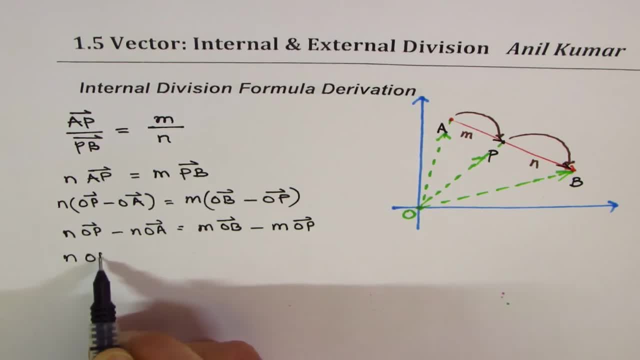 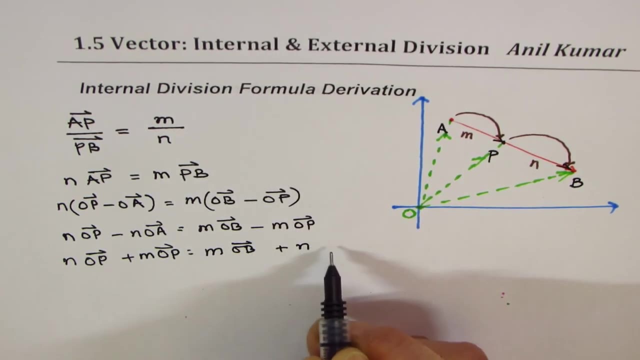 OP. Bring OP terms together: N times OP Plus M times OP equals, to take it to the right, M times OB plus NOA. Now we can take OP common, So we get. we could write this as: M plus N times OP equals 2.. 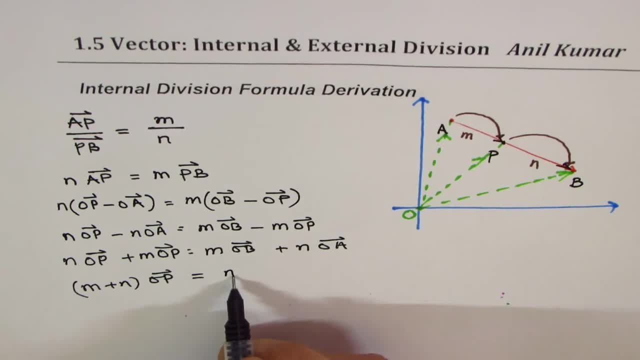 Now here we have. let me write the OA term first. So we have N times OA commutative property of addition OB. Now, dividing by M plus N, we get OP as equals to N over M plus N times OA. So we got a formula in terms of position vectors. 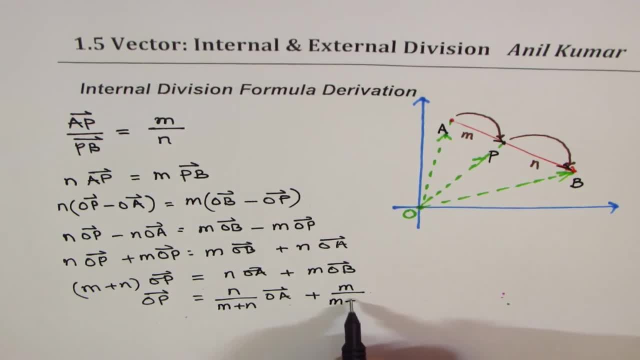 Now, that makes things very simple. So we have N times, O, B, O, B, Perfect. So that is the general formula which you can always apply to find a point P which divides a vector into two parts for a given ratio. Do you see that? 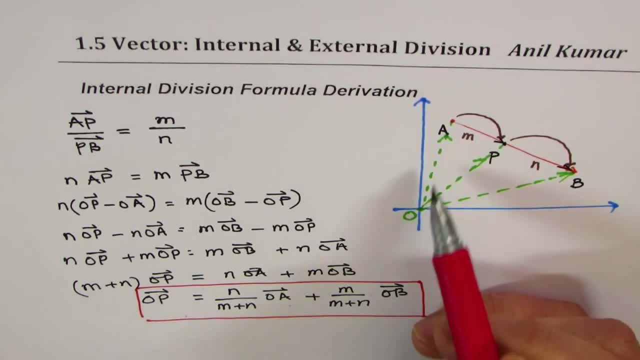 Now, if you look carefully, the term OA, the position vector OA, is being multiplied by N, divided by M plus N, by m plus n. so you can think about dividing the whole segment into m plus n parts. right, choosing n with o n and m with o p. so you get your formula, is it okay? so so if you are given, 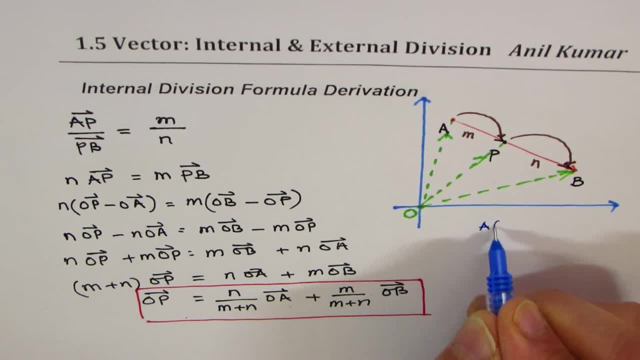 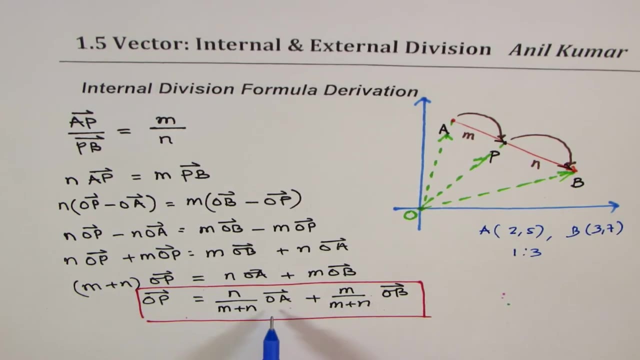 a question. let us say point a is, let's say, uh, 2, 5. let's say: and point b is 3, 7, and you are dividing it in the ratio of 1 is to 3. you can actually substitute these values here. so o, a. 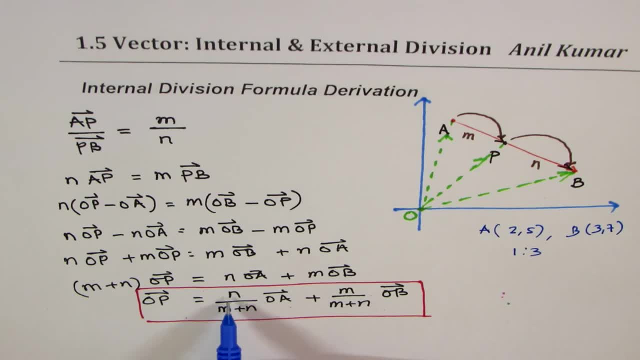 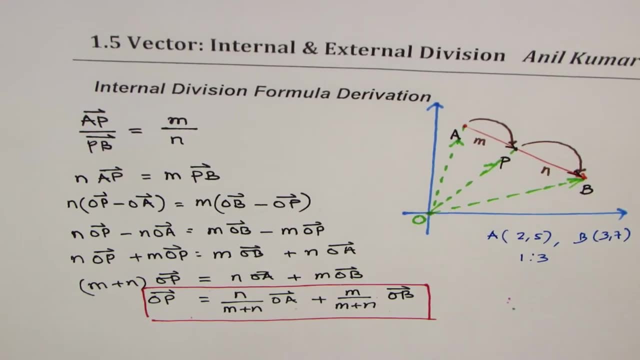 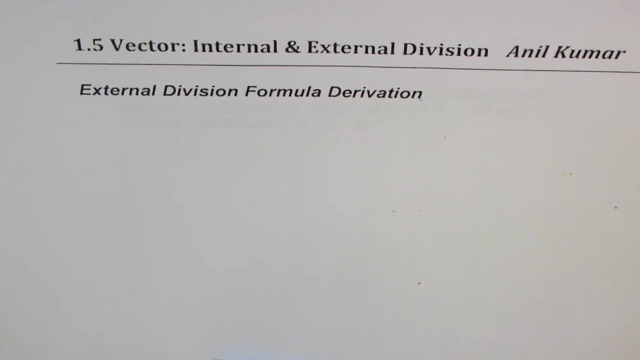 is 2, 5, b is 3, 7 and m and n are 1 and 3, and get your point b right. so that could be an exercise for you. now let's move forward and take up external division formula. now, when we are considering external division, let me again take a similar 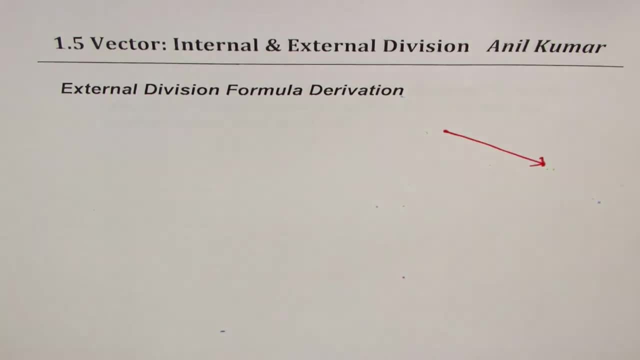 topic of an example. let's say we have a vector a, b here, but this time the point p is not between a and b, it is kind of outside collinear- collinear, but outside right. so we take a point p here. so let me label this. let's say: this is our point p, that is a and this is b. so now p is. 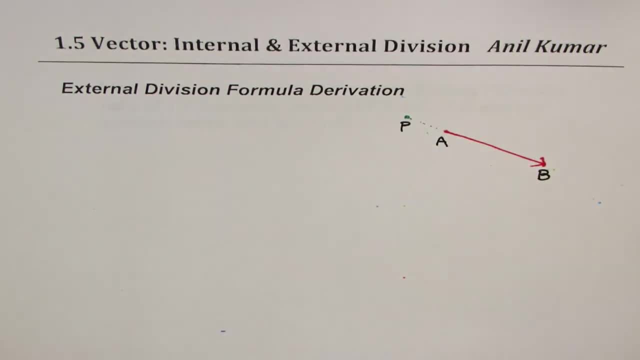 dividing the vector a, b externally. we could show it like this: so a, p will be going backwards like this, and then p, b- do you see that? so it becomes external division. so you can say that since we are going kind of backwards, we can call it external division. 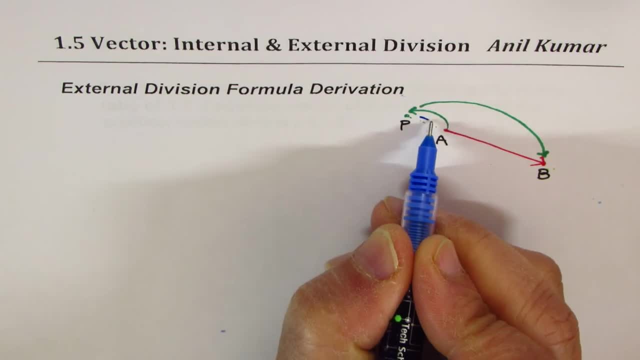 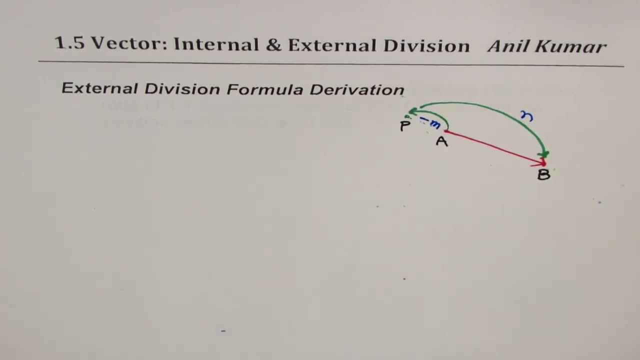 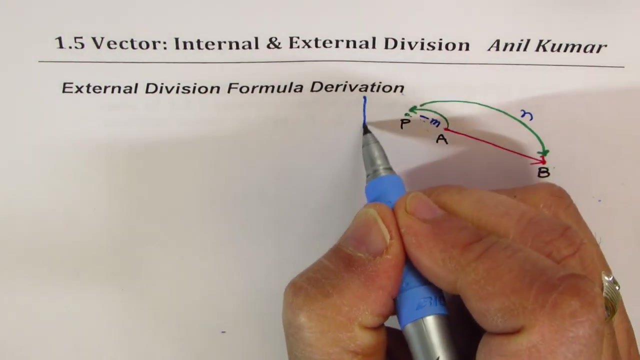 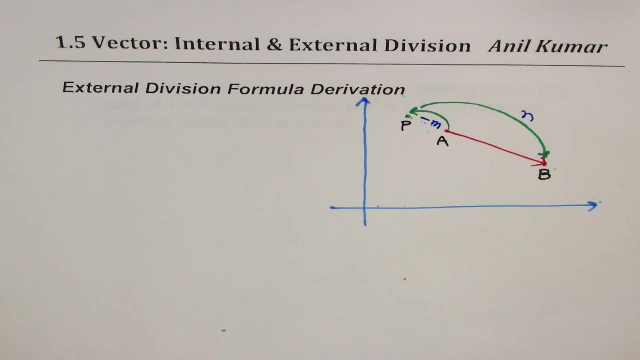 this as minus m. right, this is minus m and that becomes n going in this direction. is that all so? again, based on our coordinate plane, we'll do similar steps and derive. so consider position vectors, since normally you are given position vectors, now in this particular example, i think you can also do it. you can just pause the video. 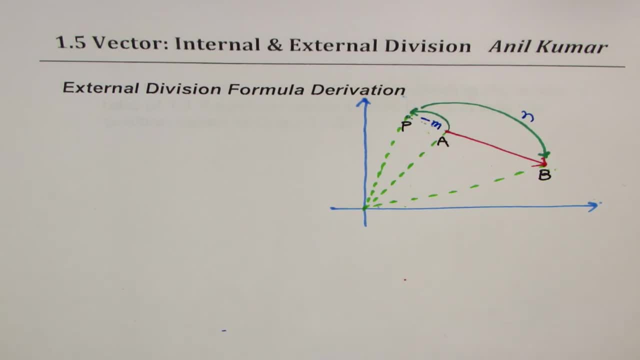 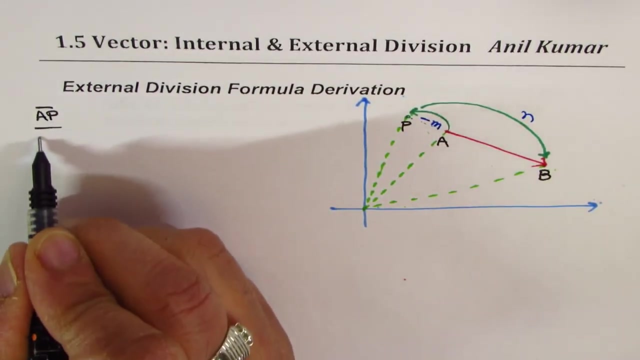 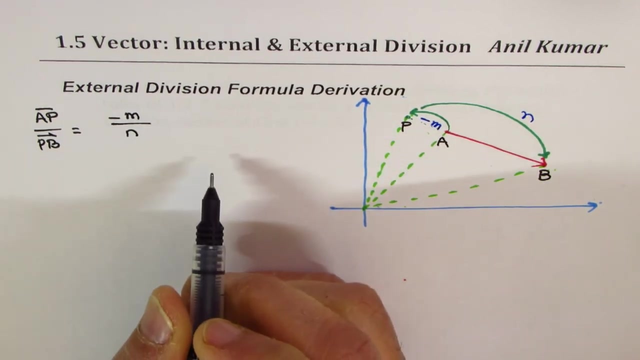 follow the steps which we did last time and check with my solution right, okay, so the strategy is a to p. the ratio a to p and p to b is given to us, which is minus m over n. okay, now we can again cross multiply. so n times a p equals to minus m times p b. 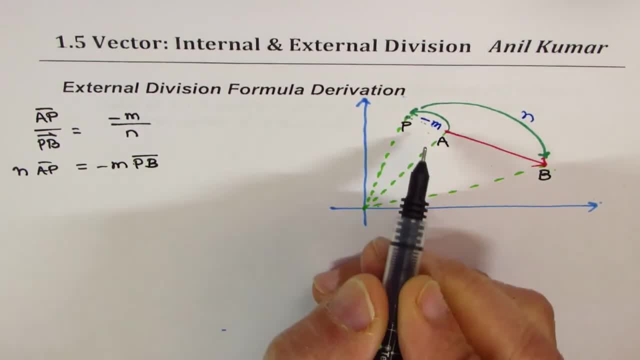 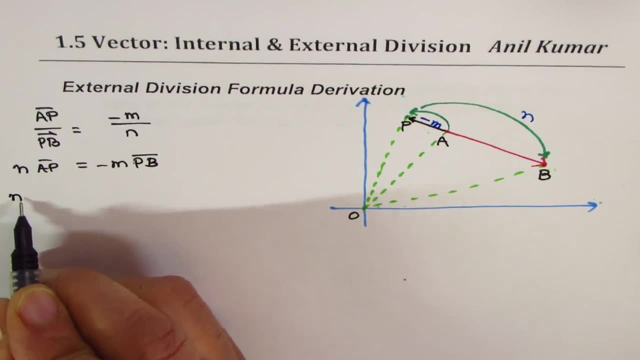 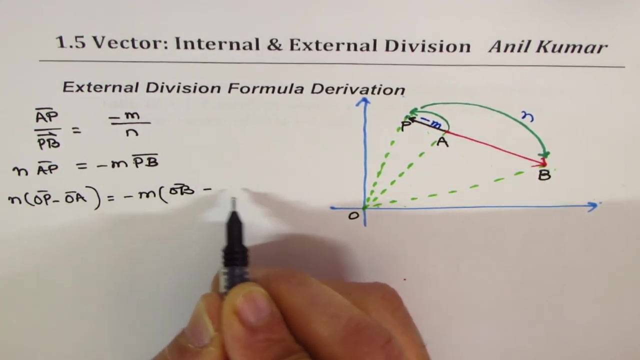 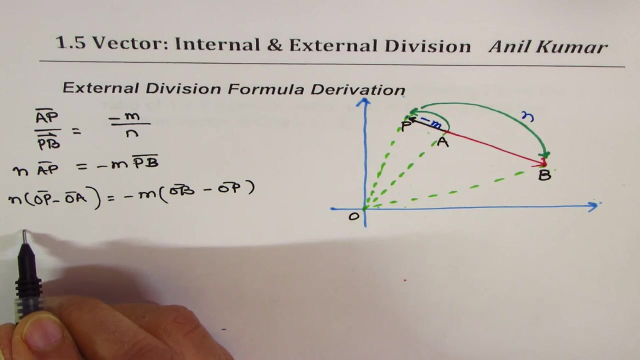 a to p. is this line right? a to p is this: that is o p minus o a, so we can write this as off. so now what we have to do is we have to get this everything written down into the bracket, all lines, and so let me make up the rest of the lambda in that square and say n minus oa. all scalar, hypertensive, evaluated here. and let's say what is this? yes, we'll do this in the next part n times estaba. okay, let's first open the bracket n times oa equals to minus m ob and let's bring how we divide blindly intoた 那 Kita, là ho, I will be able to at the last part of the bracket. here is a fraction or a fraction per Cuban. 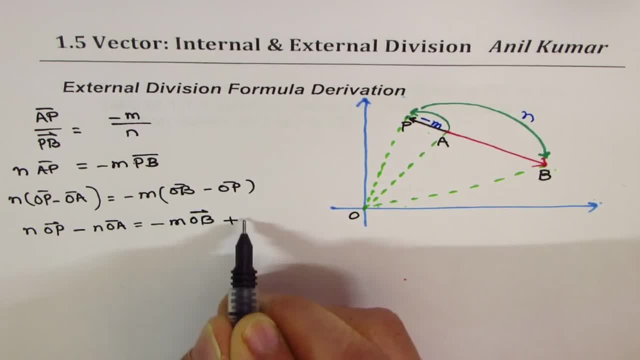 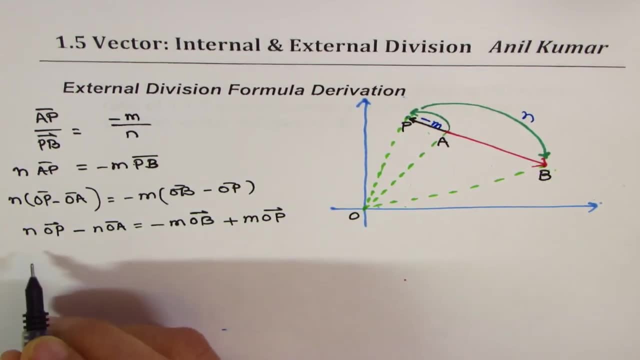 OB plus M OP. so bringing this OP term to the left, we get n OP minus M OP equals to minus M OB plus n OA. so OP is common. we can say OP n minus M equals to. now let's write OA term first: n times OA minus M times OB. now, dividing, we get OP as n over n minus M. 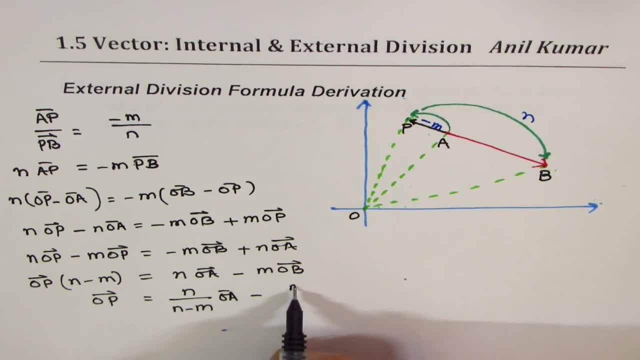 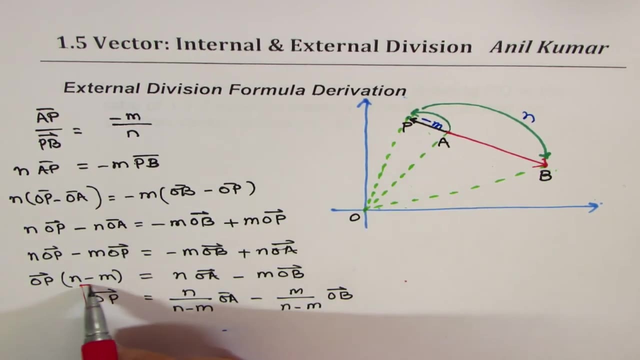 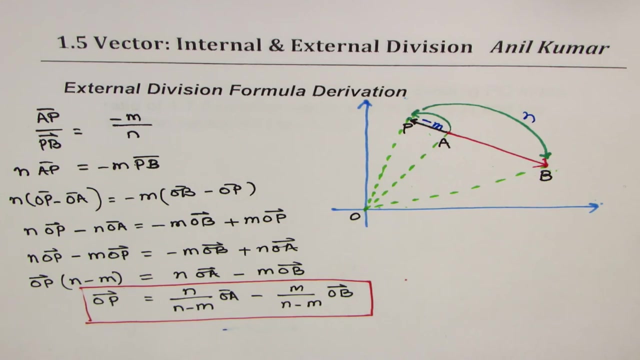 of OP, OA minus M over n minus M of OB. so this becomes our formula for external division, right? what you will notice is that the formula for internal and external actually remains same. you could replace M with minus M in your previous formula and derive the same result. so let me write here what result we got earlier. so in internal division formula. 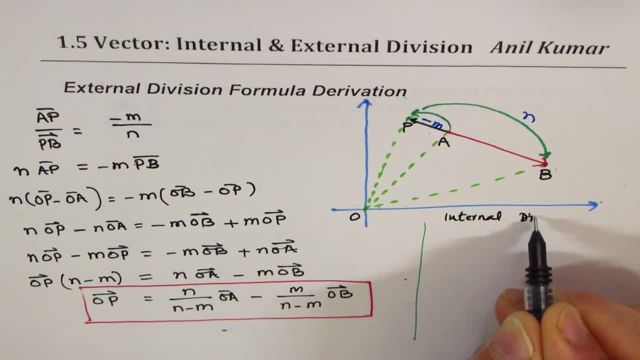 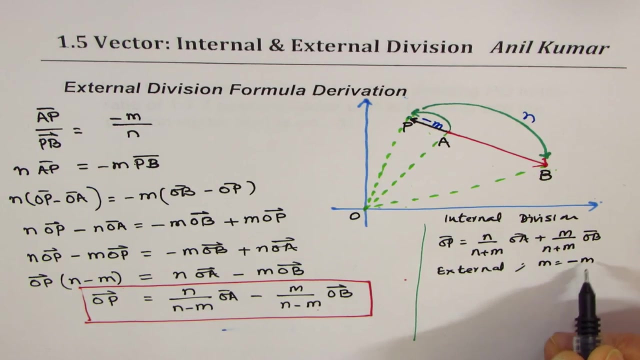 was. we got OP as n over n plus M OA plus M over n plus M OB, correct. so internal division correct. that is what we got for internal. so when we do external we replace M with minus M because it is outside. so if I do that, I get this. so you see, minus M makes this negative. 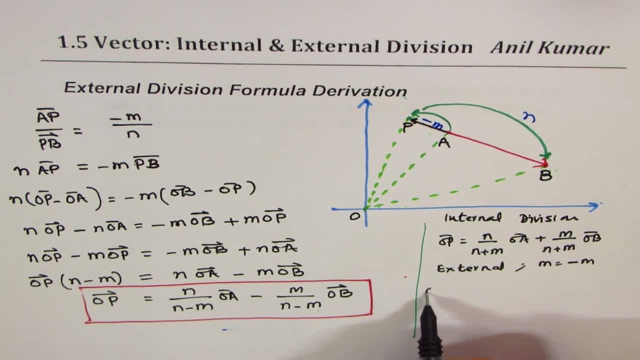 and this becomes negative. so for external OP becomes n over n minus M. so this is the formula for internal division formula. so internal division formula is enough. so we use internal division formula and make this substitution right so that becomes the substitution and you get the same result. so I hope it makes sense. perfect. so we'll take up not just the. 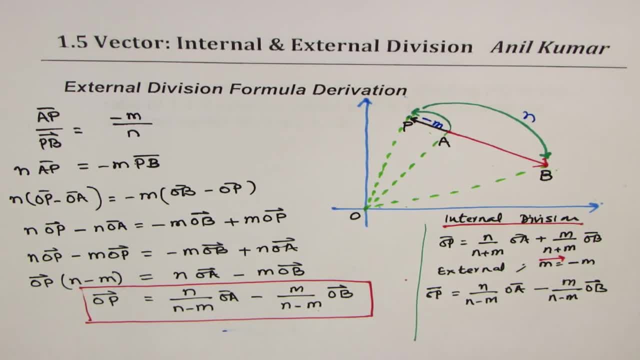 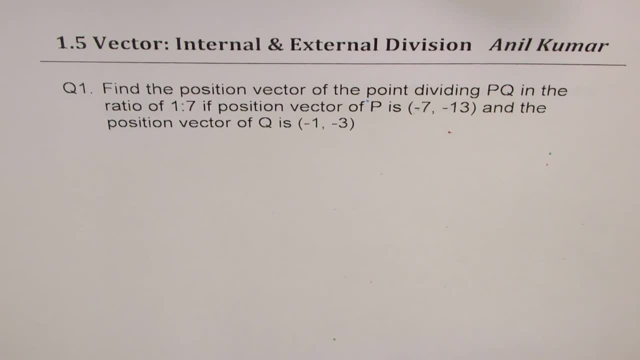 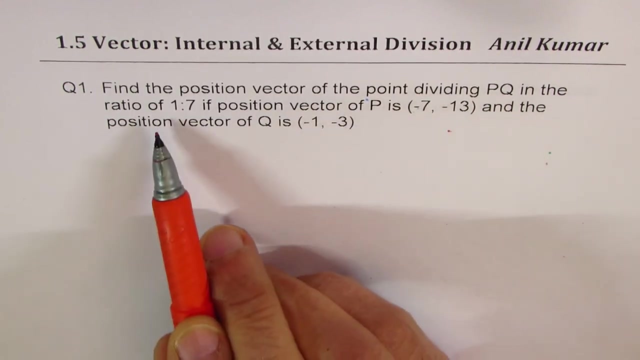 two examples apply this derivative formula and get the answers. so now let us take question number one, based on the formulas derived for external and internal division of vectors. question one: find the position vector of the point dividing PQ in the ratio of 1 is to 7 if position vectors of P is minus. 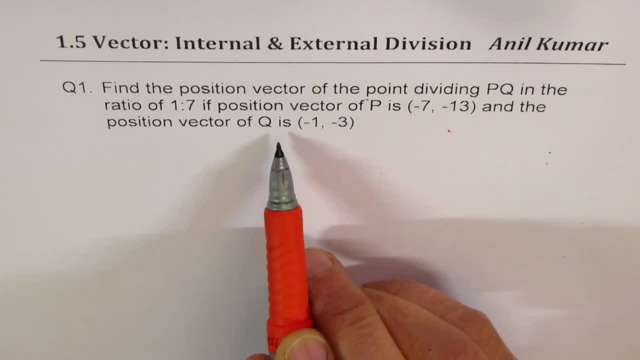 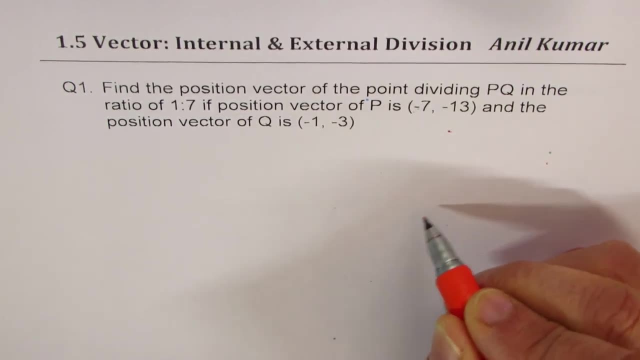 7 minus 13 and the position vector of Q is minus 1 minus 3. so so let's say we have a now something like this: alright, so that is the vector given to us where the points P and Q are. P is minus 7 minus 13 and point Q is minus 1 minus 3, right? 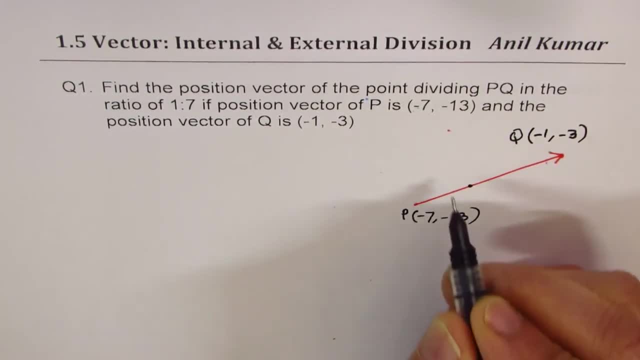 we are looking for a point somewhere in between, let's say, r which divides pq, which is this point in the ratio of 1 is to 7. so so what we are looking for is that this is from here to here is 1 unit and from here to there is 7 units. right, 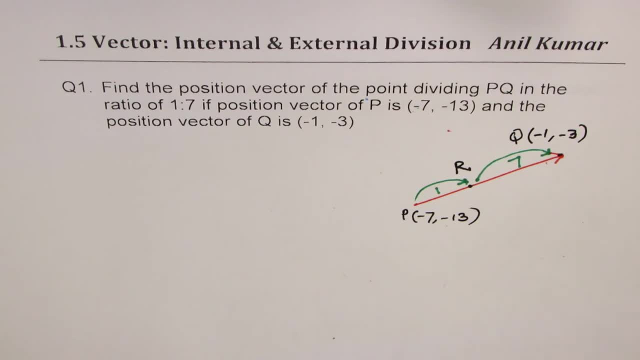 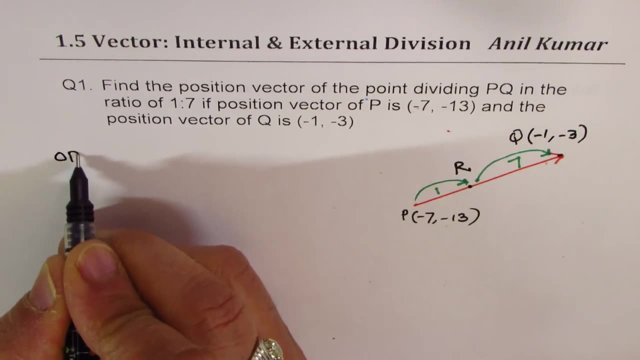 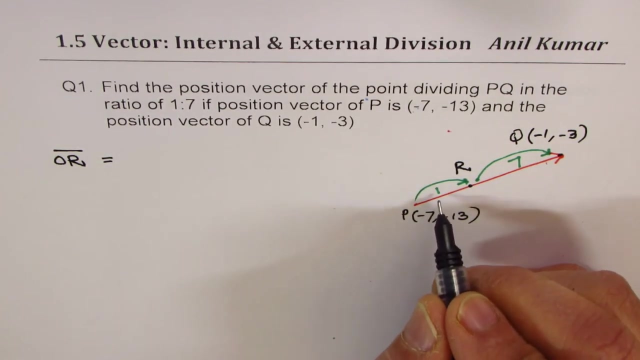 so that is what we are looking for now. we have derived this formula and we know that the position or so, or gives you the position vector- is equal to now. if i treat this, this is one right. so the formula is: let us say: if i write this as n, let me write down. let me write down the formula. 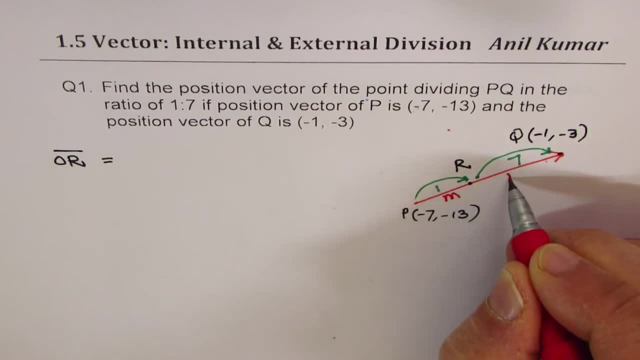 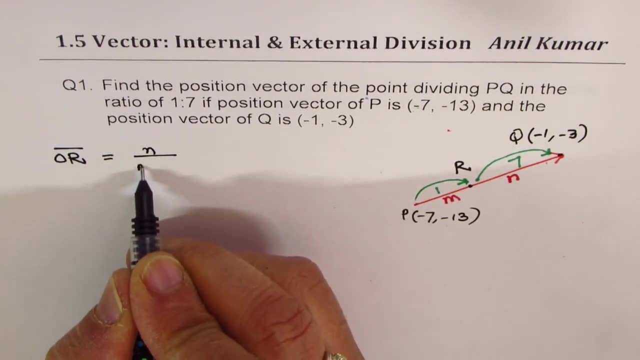 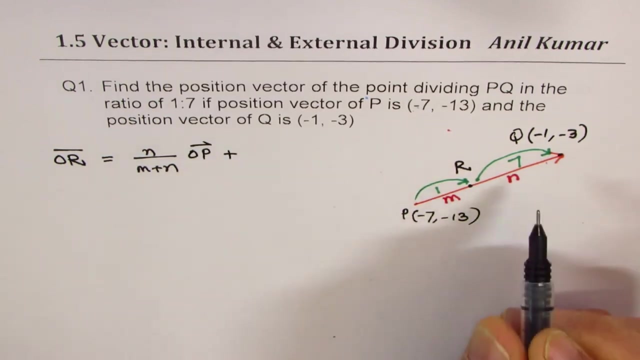 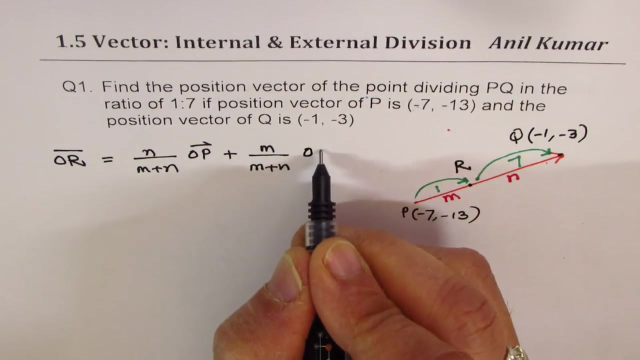 with respect to what we did. if i write this as m and this is n, in that case the formula is n times r, r, r and over some of these two m plus n times op right plus m over m plus n times oq. that becomes the formula, is it okay? 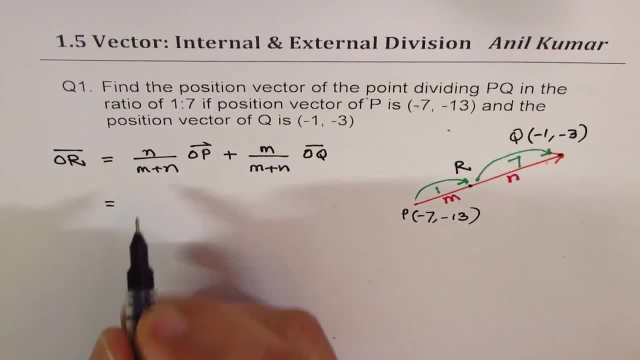 so, or in our case, n is 7, so we get 7 over 7 plus 1. op is minus 7 minus 13, so minus 7 minus 13 plus m over mn, that is 1 over 7 plus 1, and oq is minus 1 minus 3. is it okay? 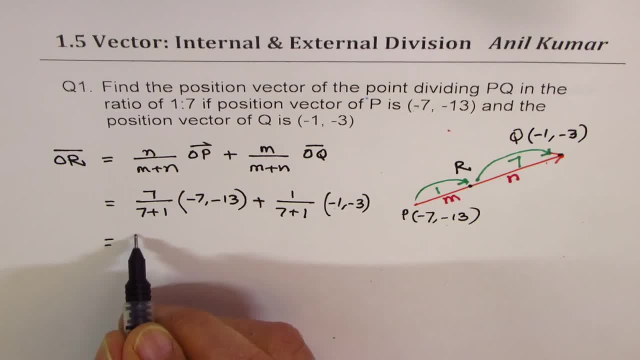 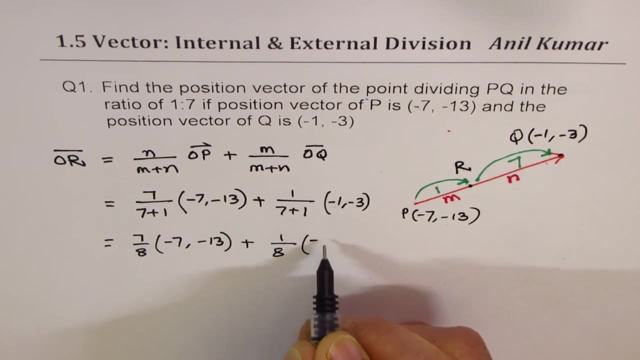 so what we get here is 7 over 8 times minus 7 minus 13 plus m over mn, that is, 1 over 7 plus 1, and oq is minus 1 minus 3. is it okay? minus 13 plus 1 over 8 times minus 1 minus 3, right? 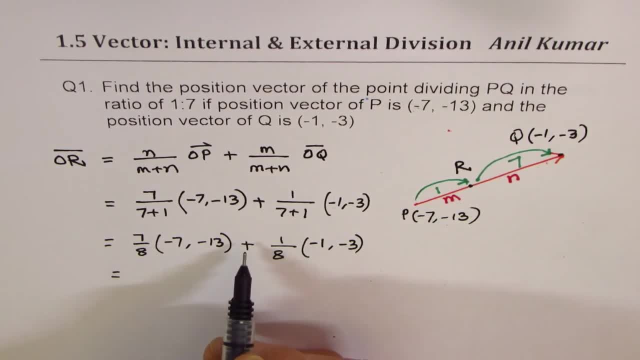 so when you add them, you add the corresponding x and y values. so what you get here is 7 times 7, is 49 over 8 plus this, which is minus 1 over 8. so that becomes the x coordinate. and as far as the y coordinate is concerned, 7 times 8 is minus 6. and visiting ます會. 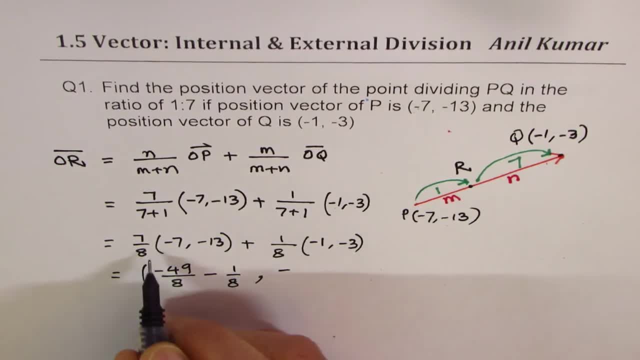 y beliefs. concern of this will solve the problem here, isn't it okay? times 13,, which is negative, 7 times 3 is 21,. 2, 91, divided by 8, and minus 3 over 8, right. 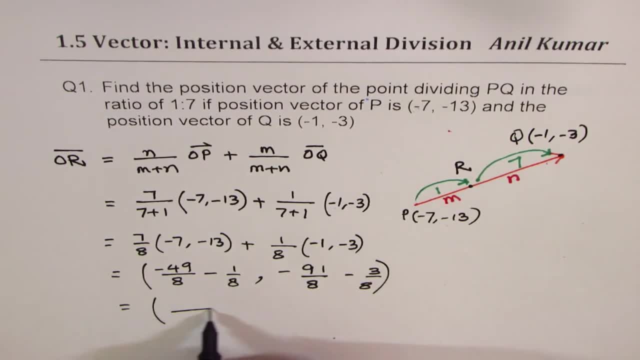 So the position vector is 8, and when you add this it becomes minus 50, and here it is minus 94 over 8.. So that becomes the position of R. So the position vector is this. Do you get an idea? 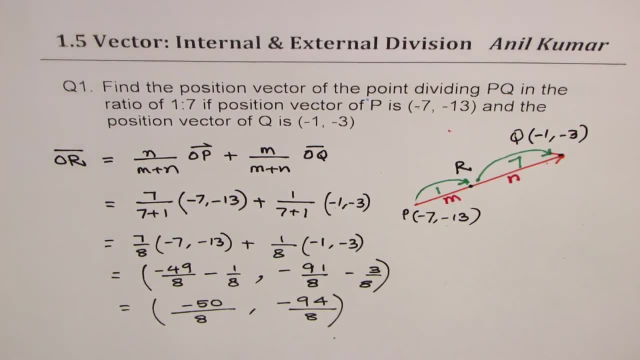 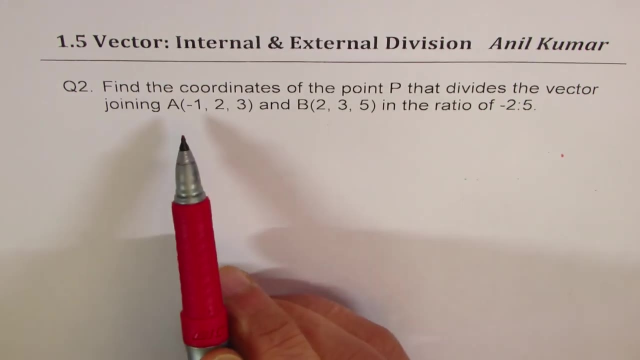 That is how it can be solved. So it really helps to remember the formula and do such questions. You could have derived it also. okay, Now let's take an example on external division also. So in this case we are working in R3.. 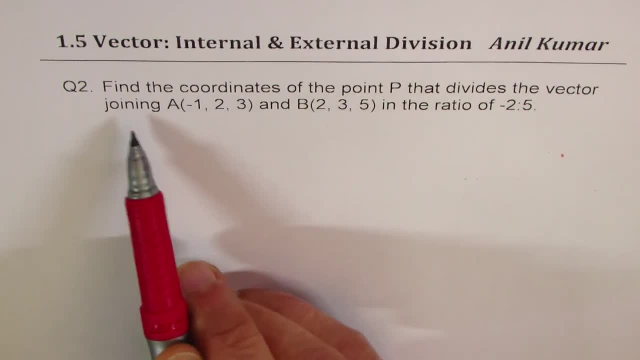 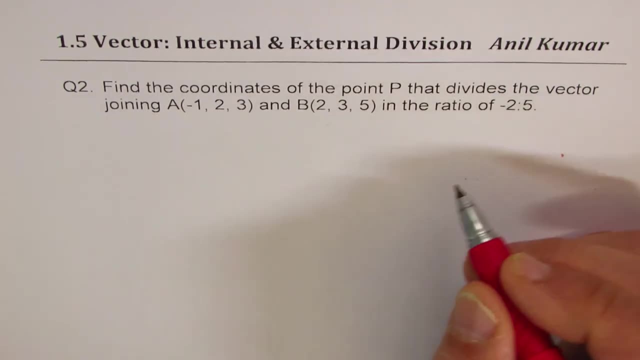 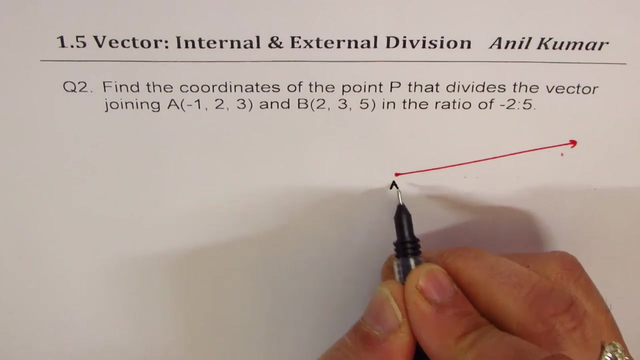 Find the coordinates of point P That divides the vector. joining A and B in the ratio of minus 2 is to 5.. So let me just randomly just draw the vector from A to B, where coordinates of B are 2,, 3,, 5, and that of A are minus 1,, 2, 3.. 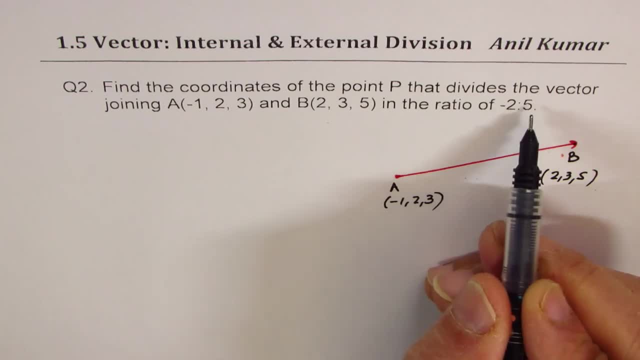 When we say, divide The points in this ratio of minus 2, that means PA is this side right. So we are doing AP right. So the point is outside. So basically it means that the point is somewhere here. 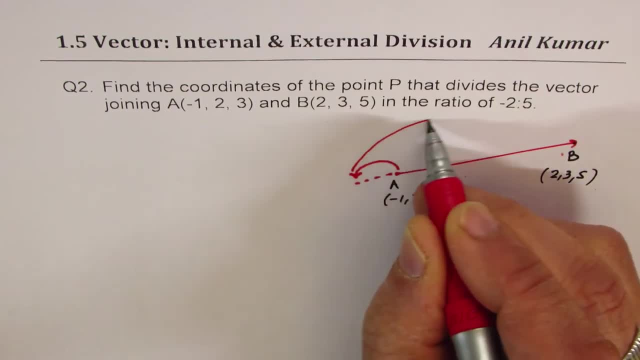 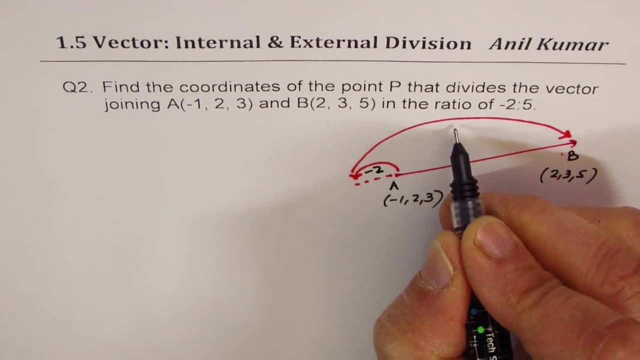 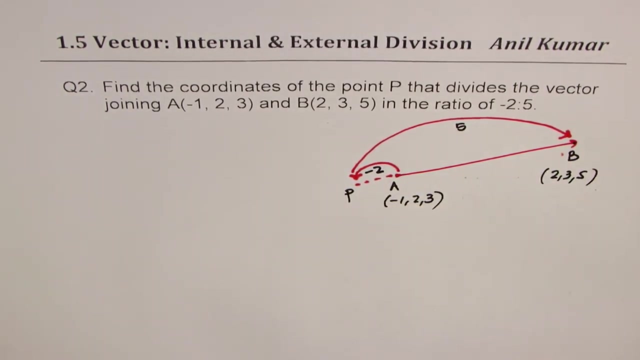 So you go to this side first and then there You get an idea. So that is minus 2.. This is minus 2, and this is 5 for the point P, which is collinear with AB. However, it is external to the vector AB. 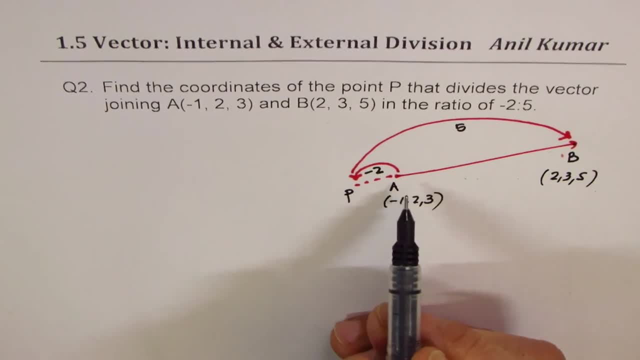 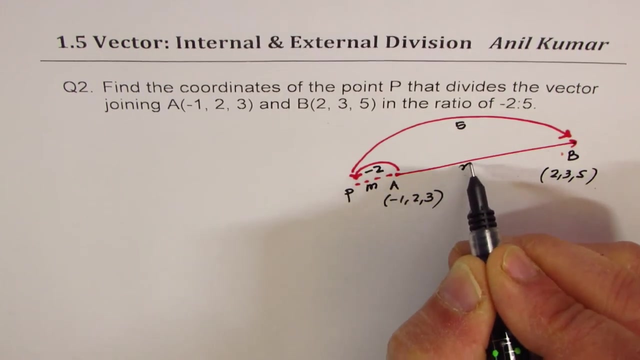 So I hope that makes sense. right? So we'll actually use the internal formula, but use negative 2 instead. right? So the formula is, if I'm using this section, as in general, if I write this as, let us say, M, and this is as N, right? 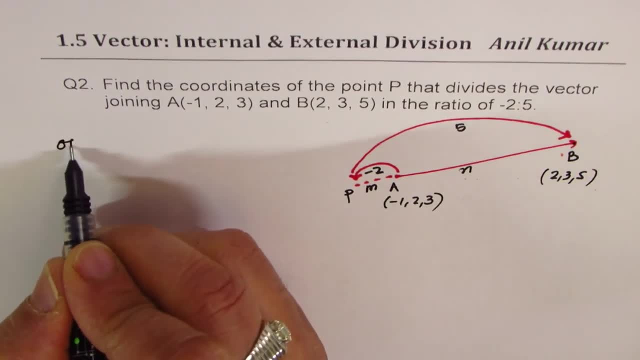 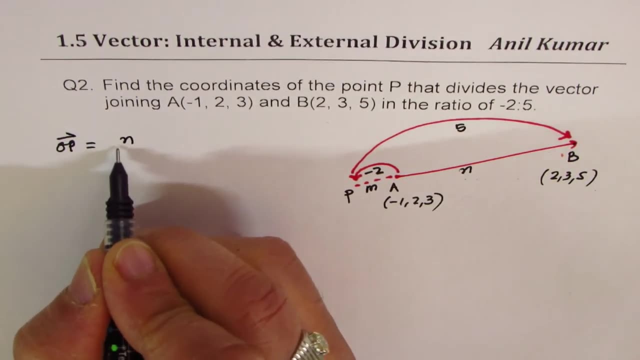 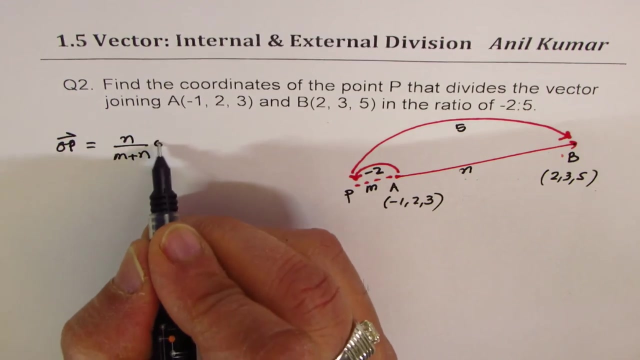 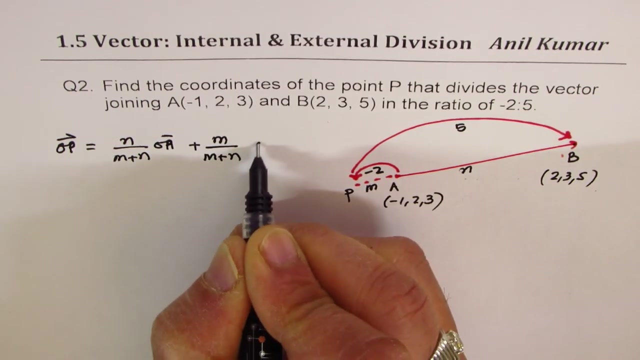 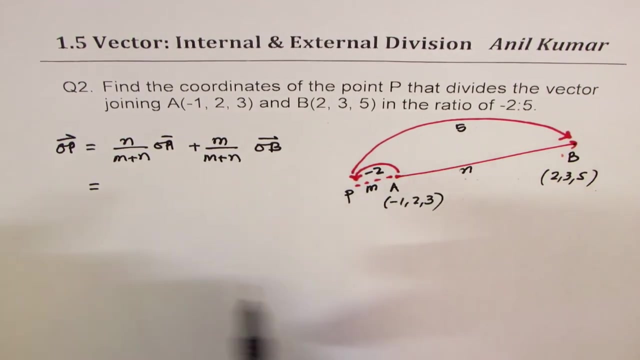 So we say OP is Position vector. OP is equals to N over M plus N times OA plus M over M plus N times OP. Perfect, Now, in our case N is positive 5.. So we write 5 over. 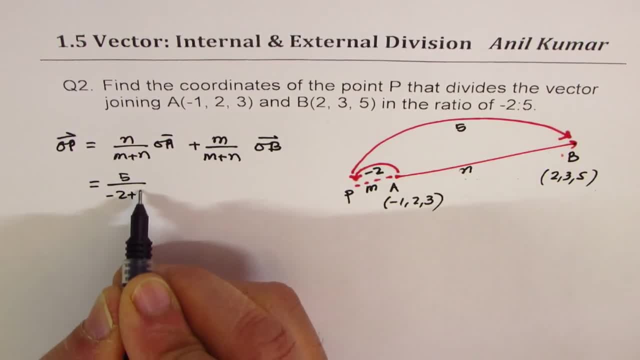 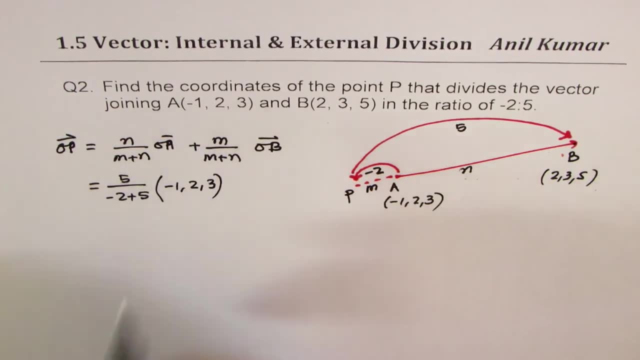 Then we have minus 2 and 5.. Minus 2 plus 5, right And coordinates of OA are minus 1,, 2, and 3.. Directly you get the value from here: right Plus M is minus 2.. 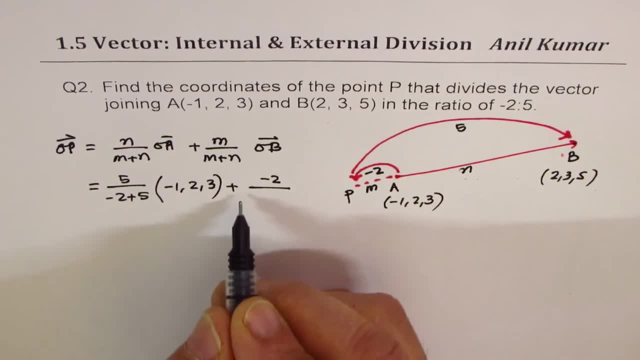 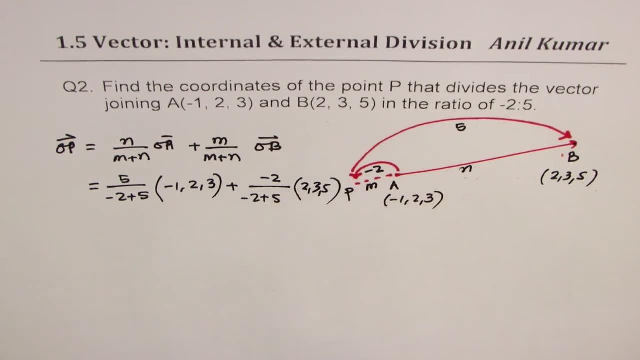 So I'll write minus 2 here, divided by minus 2, plus 5 times the coordinates of B, which are 2,, 3, 5.. You get an idea right. So that is how it should be done, right. 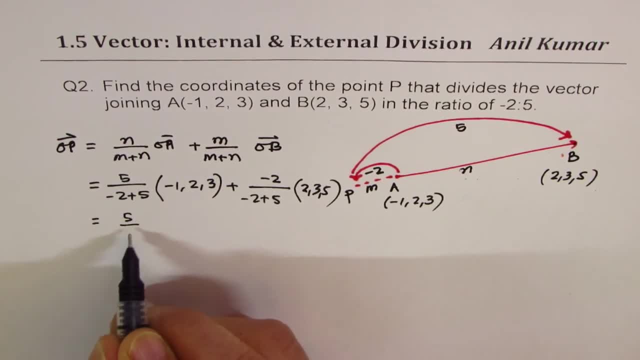 So So you could write this as 5 over 3.. Now let me write these formulas in vertical form: Minus 1, 2, 3.. That's another way of writing the same thing, right? Minus 2 over 3.. 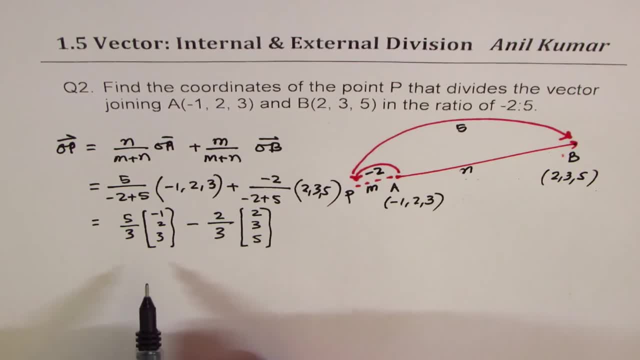 2, 3, 5.. It becomes simpler if I show you like this. So basically, when you add this up, you get minus 5 over 3. And when you multiply this, it is minus 4 over 3, right. 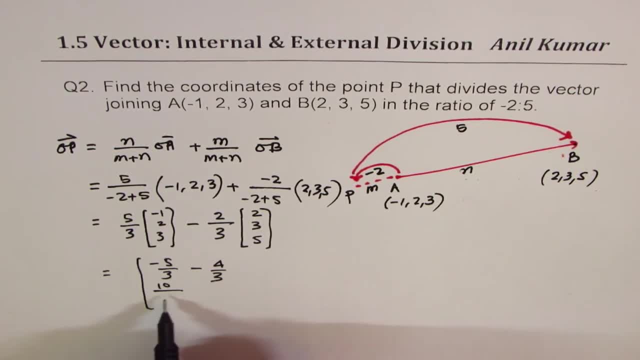 And then we get 10 over 3, okay, 10 over 3, minus 6 over 3.. Minus 6 over 3.. And here we get 15 over 3. And we get minus 10 over 3.. 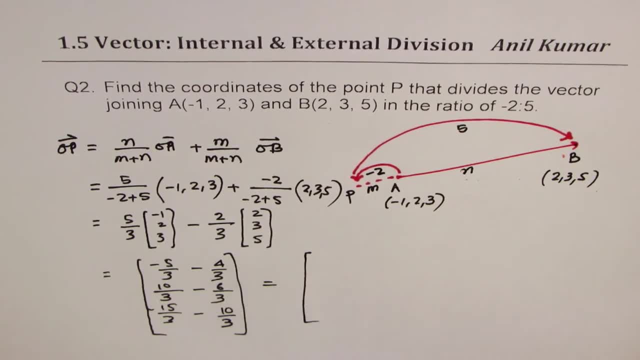 So the position vectors are minus 9 over 3.. This gives you 4 over 3.. And that gives you 5 over 3, okay, So that becomes the position vector of OP. So our answer is OP. 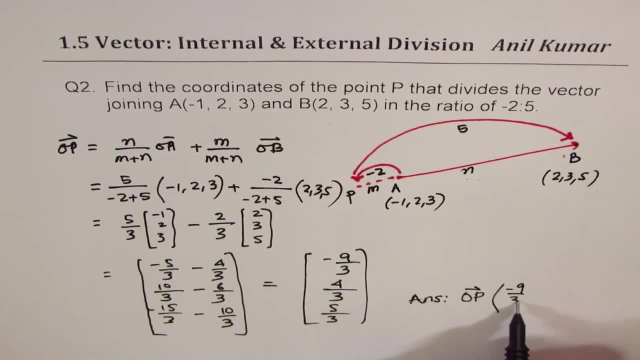 Position. vector OP is minus 9 over 3,, 4 over 3, and 5.. So I hope the concept is absolutely clear so you could easily find a point. which divides a vector internally or externally in a ratio of m is to n. 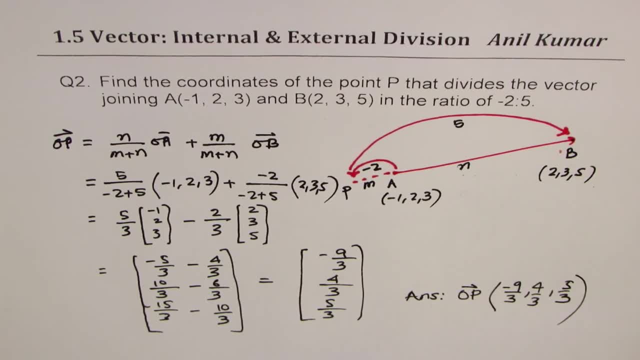 Feel free to write your comments and share your views and, if you like, and subscribe my videos, that would be great. Thank you and all the best.